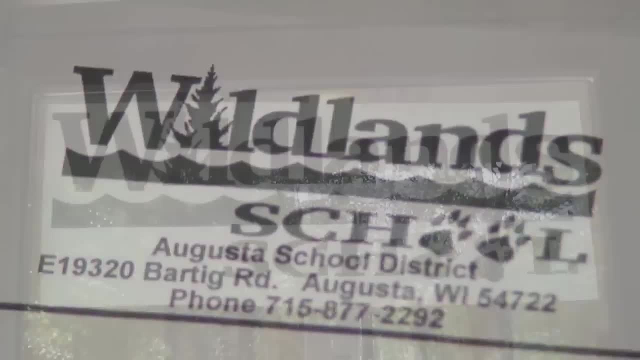 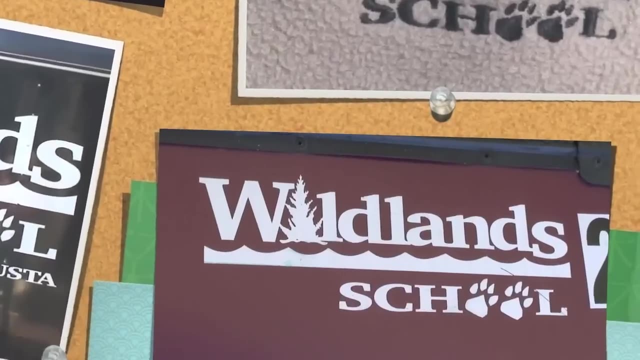 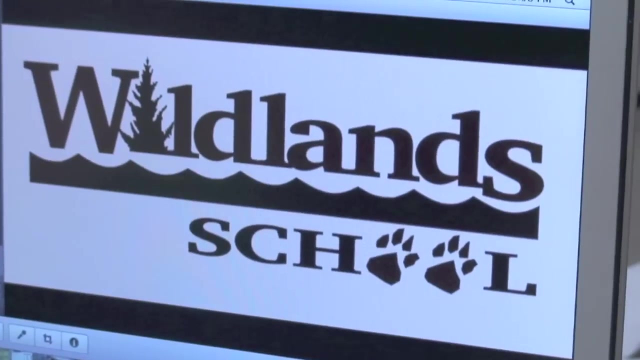 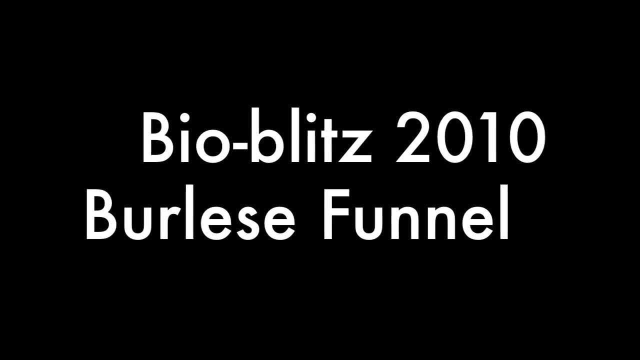 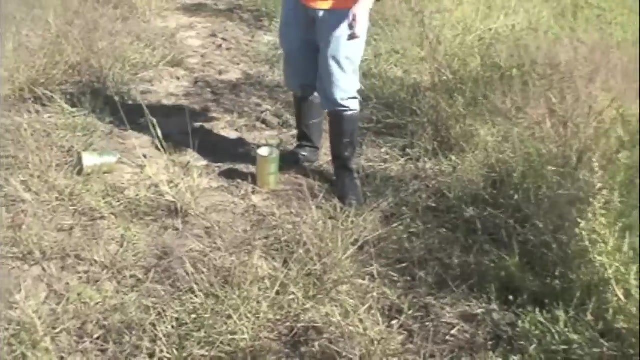 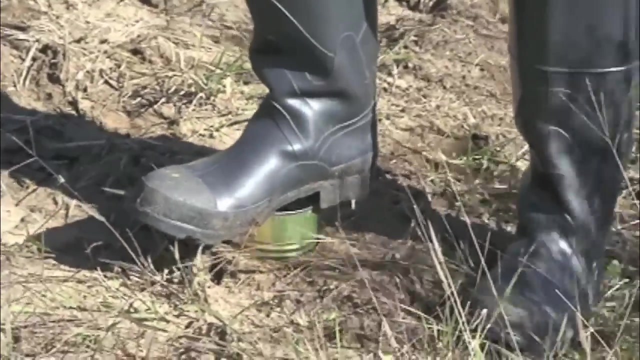 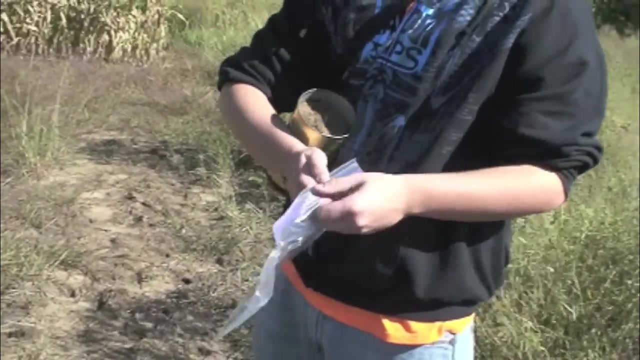 One way to take a soil sample is to take: Take a coffee can with the bottom, cut out and press it into the soil, applying equal pressure to the top of the can. Using two hands, pull the can out of the soil and place the can with the soil into a 1 gallon. 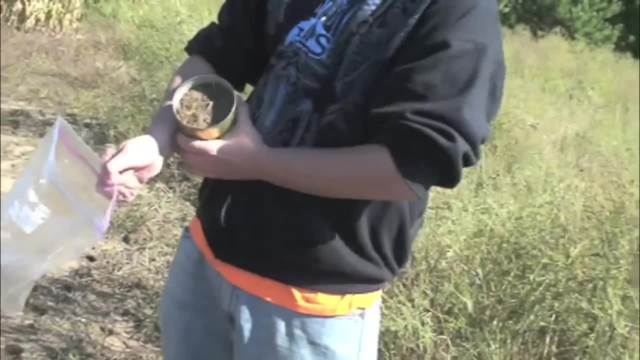 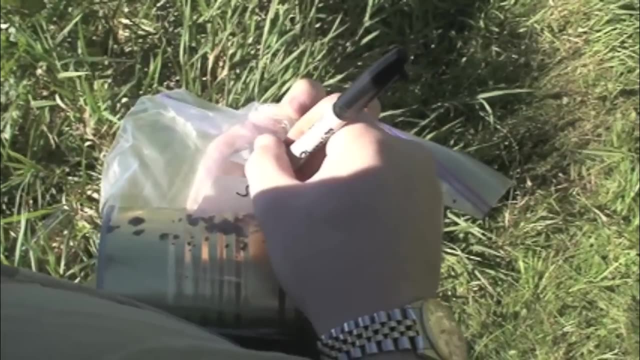 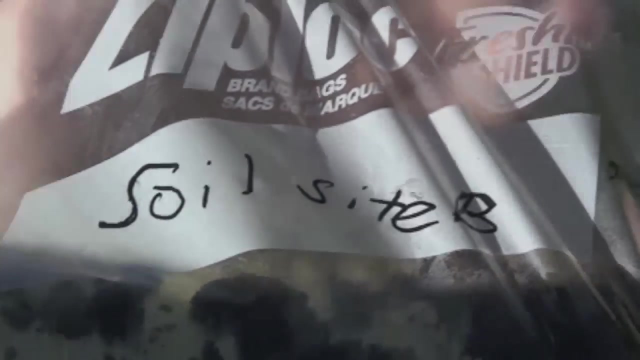 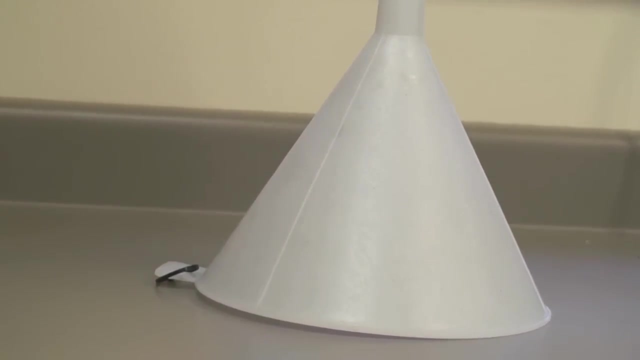 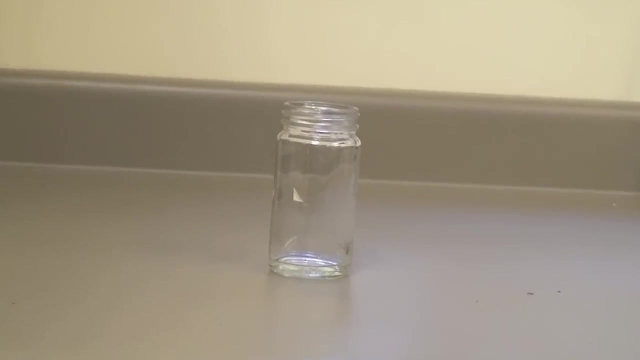 plastic bag. Make sure to seal your bag tightly and label the bag with the location you took the sample from. To make a Burley's funnel you need to acquire a funnel that can fit one full soil sample. You will need a jar with 1 quarter cup of ethyl alcohol. 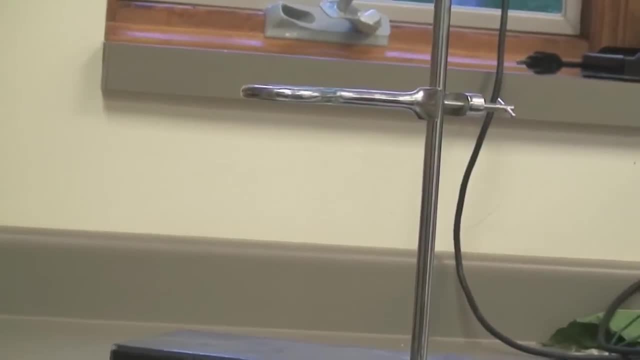 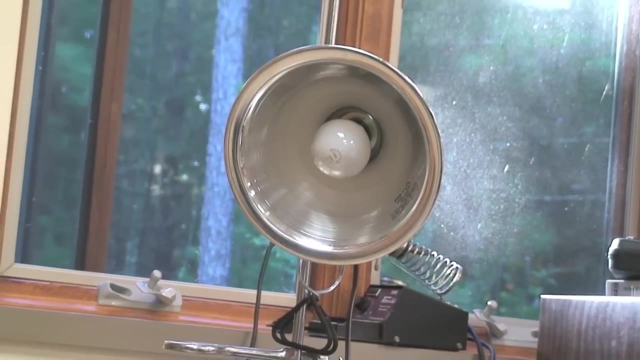 You will also need a sturdy ring stand. Make sure to seal your bag tightly and label the bag with the location you took the sample from. The last item you will need is a heat lamp. Place the jar of ethyl alcohol underneath the funnel. 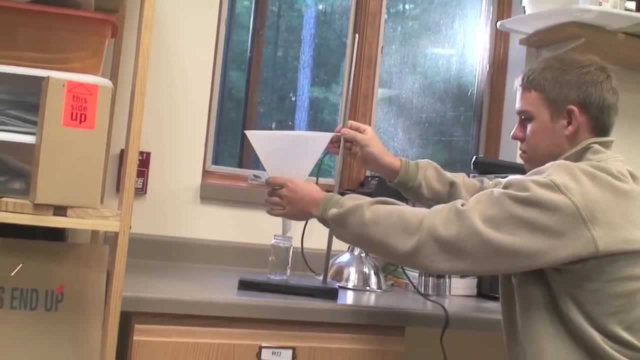 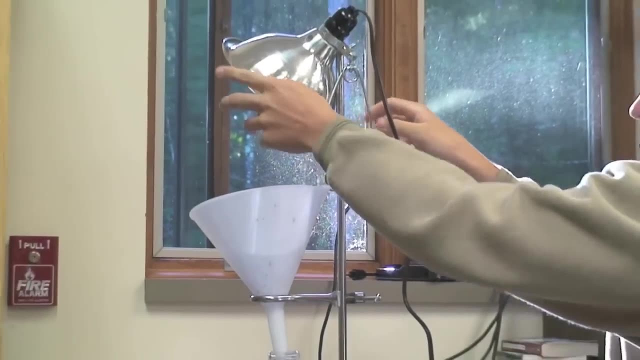 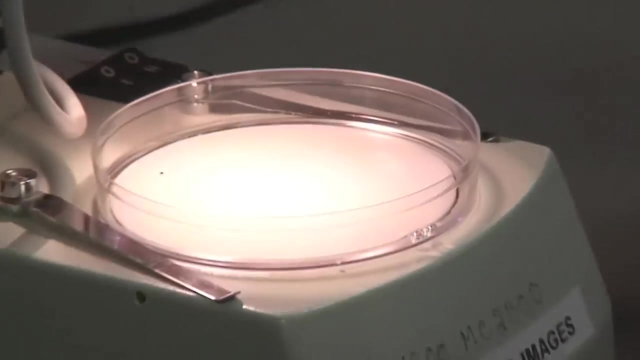 Attach the funnel to the ring stand. Clamp the heat lamp to the top of the ring stand. Angle the heat lamp towards the top of the funnel. Dump the soil sample into the funnel. Pull the funnel out of the funnel. Take out the soil sample. 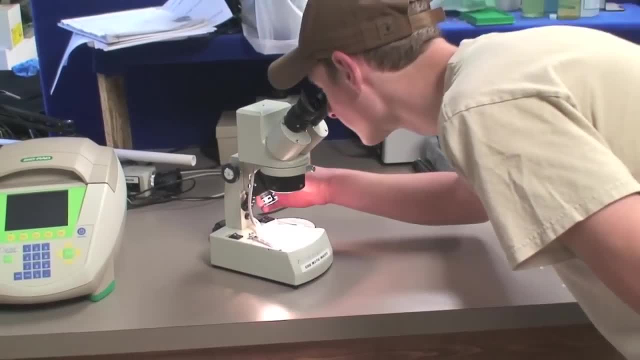 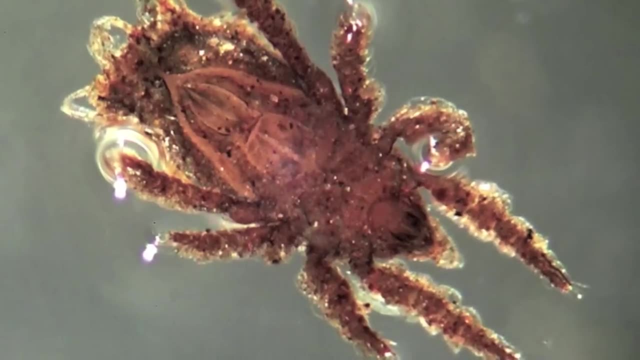 Remove the soil from the jar. Let the soil end of the funnel stay inside the jar for about 5 minutes. After 3 days, remove the soil insects from the jar of ethyl alcohol and examine them underneath a microscope. The reason the soil insects fall into the jar of ethyl alcohol is due to the fact that